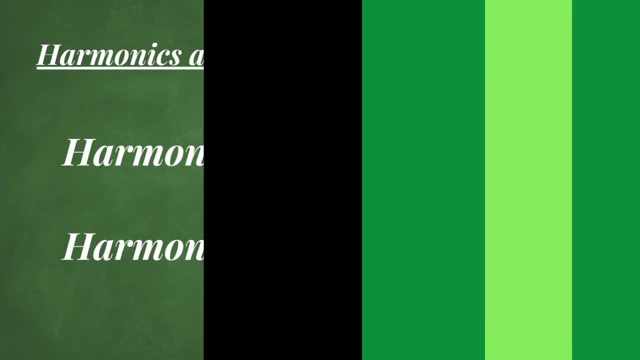 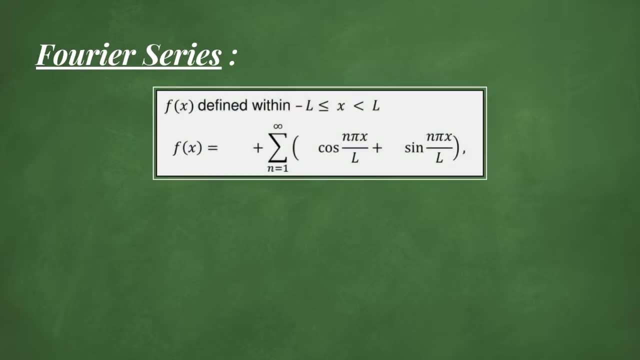 whereas the opposite isn't the case. Okay, now on the technical side. the Fourier series is a summation of harmonics, so cosine and sine functions having a frequency that increases each time the number n increases, We have to introduce some coefficients, a and b, in some way to adapt them to our function f that we want to approximate. 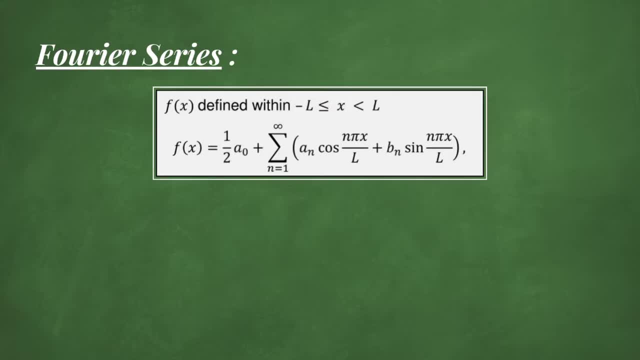 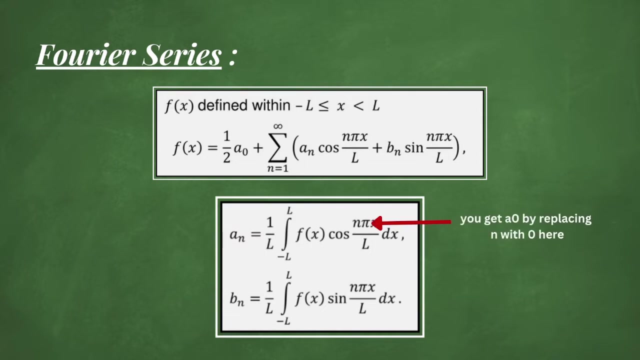 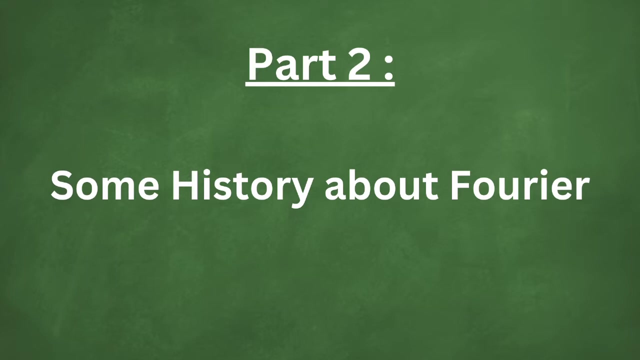 So here we go. These coefficients are obtained by evaluating this formula, so by integrating our f function- times cosine for a and then times sine for b- across the periodic domain, whereas a0 is obtained just by integrating our f function. Now, before we can move on, let's take the time to talk about Siri Fourier himself and do some. 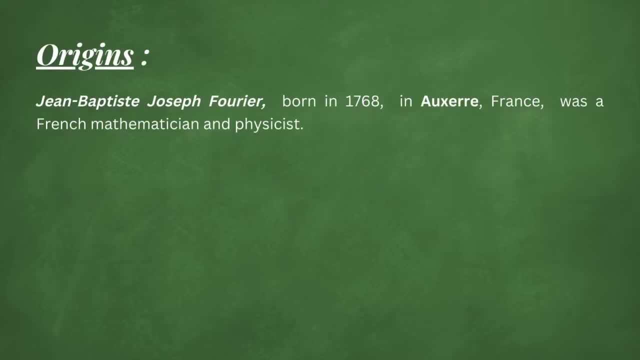 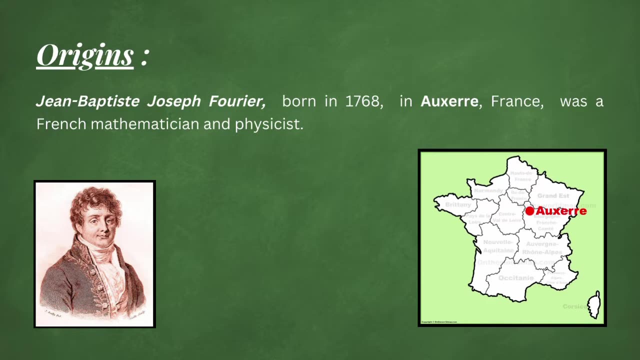 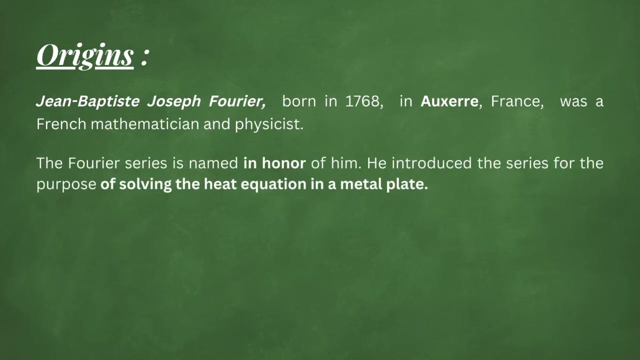 high school chemistry. So Jean-Baptiste Joseph Fourier, born in the 70s in Auxery, France, was a French mathematician and physicist. The Fourier series is named in honor of him, where he introduced the series for the purpose of solving the heat equation in a metal plate. So it was the problem he was working on at. 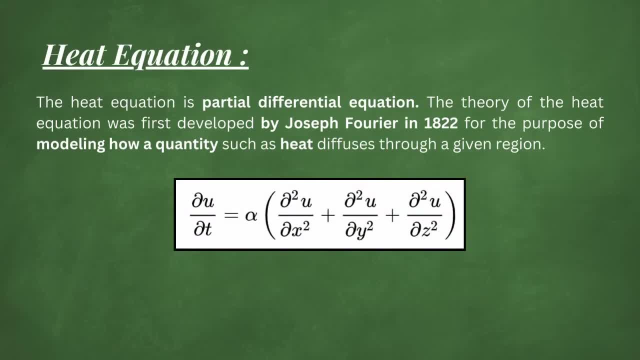 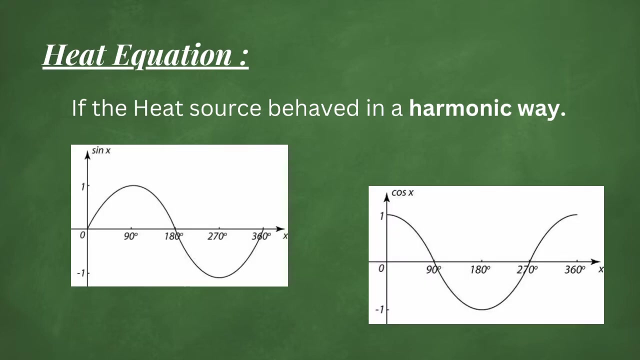 that time. Now the heat equation is a partial differential equation. Prior to Fourier's work, no solution to the heat equation was known in the general case, although particular solutions were known if the heat source behaved in a simple, harmonic way, so if the heat source was a sine or cosine. 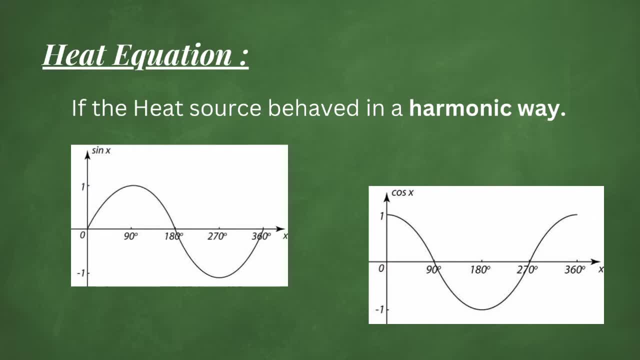 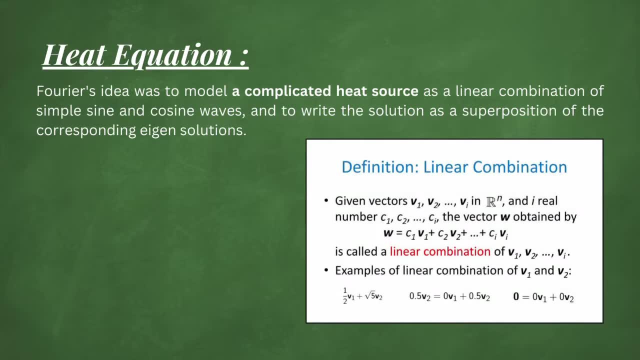 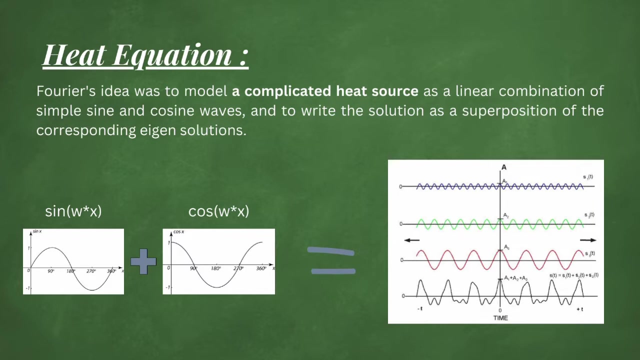 wave, which isn't really the case in the real world. Fourier's idea was to model a complicated heat source as a linear combination of simple sine and cosine wave and to write the solution as a superposition of the corresponding eigen solutions. The superposition, or linear combination, is called the Fourier series. 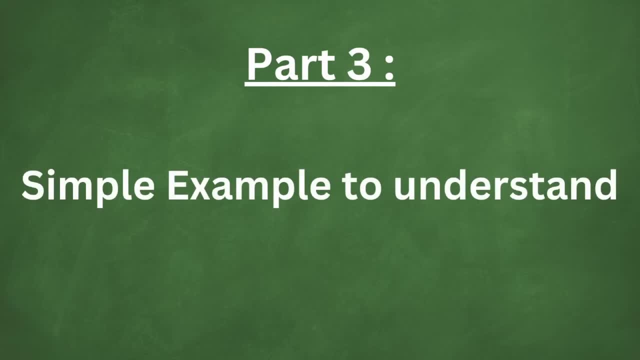 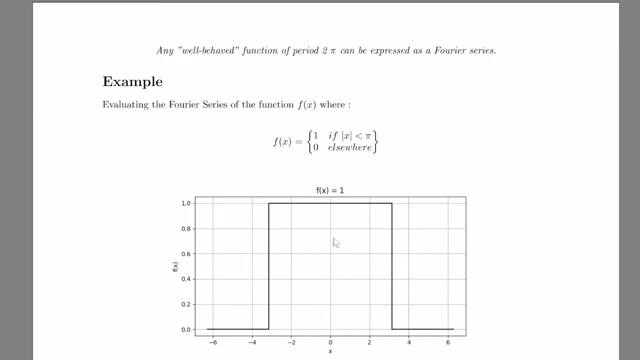 Now let's take a quick and easy example to evaluate a Fourier series. Okay, So let's say we have this function right here, which is equal to one if x is less than pi and it's equal to zero elsewhere. So the first thing we got to do is to compute the terms, the a and b terms. 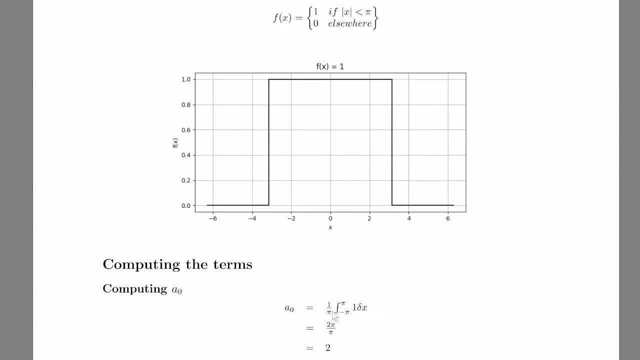 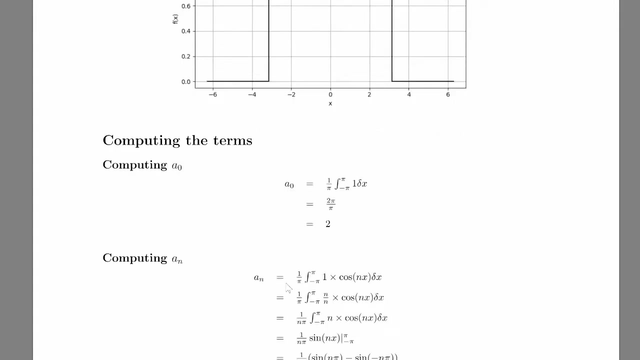 Here we can simply compute a and zero, which is equal to two directly, because f is equal to one, and then you integrate it. it gives two pi. then two pi over pi is equal to two, and then we compute the a, n. So this is also equal to one times cos n of x, and then we integrate it. you get this and 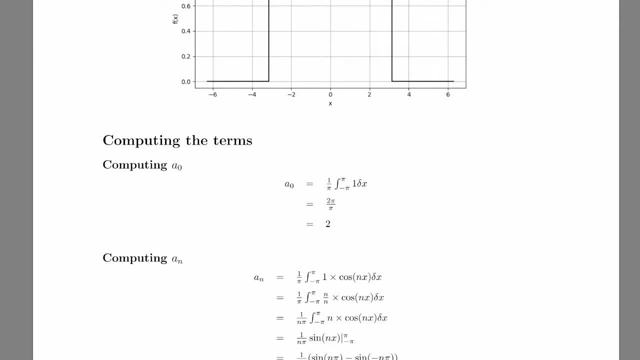 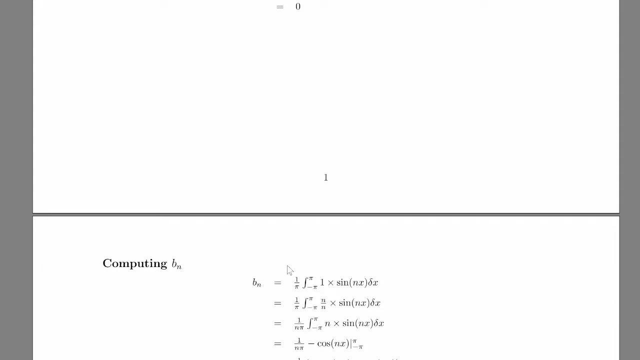 then this results in this expression right here, which is equal to zero all the time, because sine of n, pi is always equal to zero, and this is also always equal to zero. So it's zero minus zero, which is zero as well. And then it's also the same for b? n. 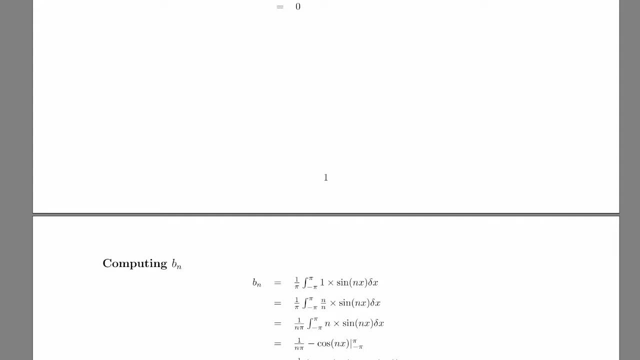 We integrate it, and then we evaluate it, and so on. We get zero as well. All right, So this is a bit expectable, because our function is even So. you have f of x is equal of f of minus x, which is equal to one, and then we get this: 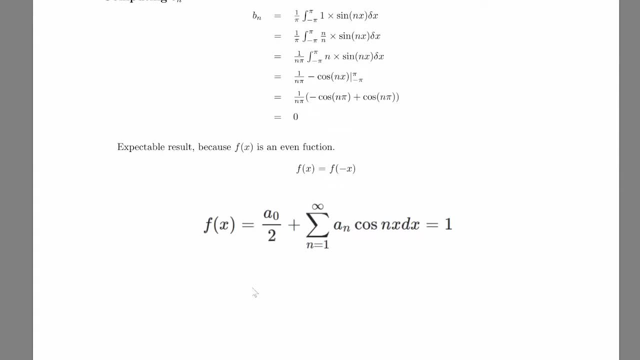 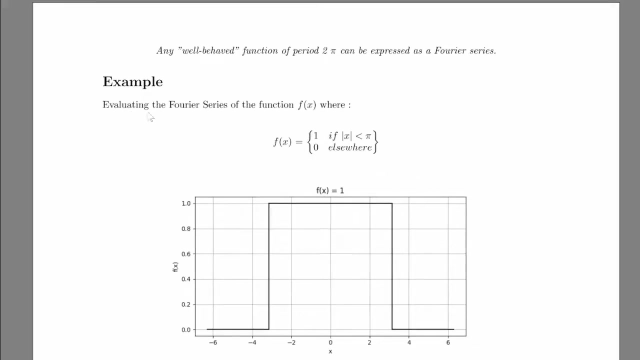 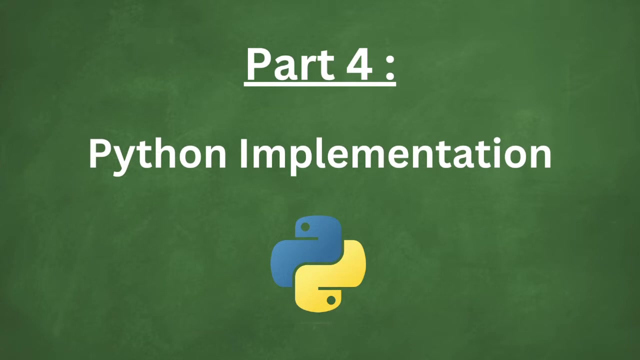 result. Okay, So this is kind of a very simple and basic example, but it is an example with which you can better understand what is happening in the series. Okay, Now the last thing to do is to go in Python and try to implement this method. 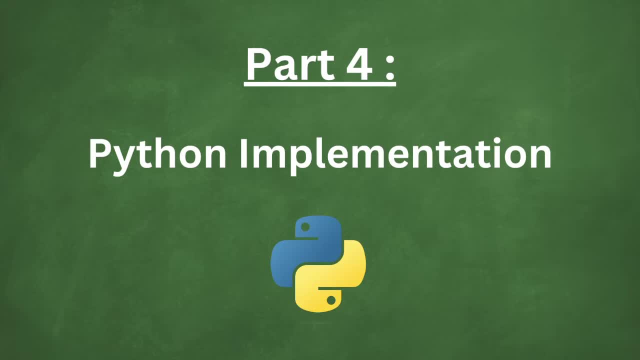 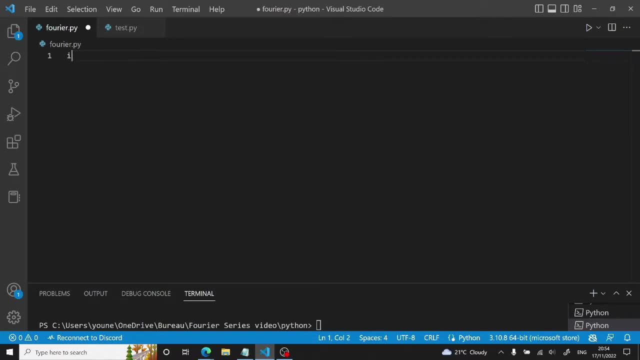 So I'll see you in my Visual Studio code, Okay. So here we are in our Visual Studio code interface and we will start by importing our numpy module, as always, Okay, And we will define our periodicity, which will be l, Let's say it's equal to nppi. 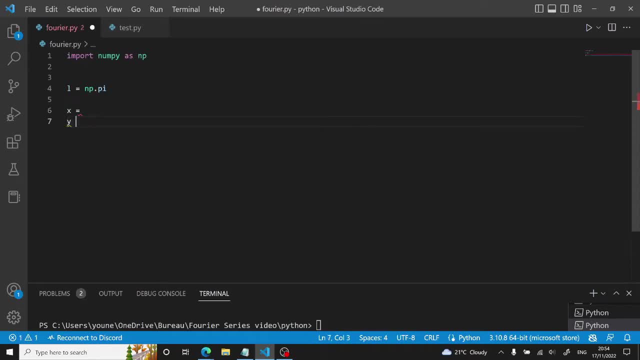 Okay, Now we will create our x and y vector, So x will be equal to numpylit, Okay, And then we will create our bin space, like: so It will start from minus l and in l across, say, 500 values. So this will generate a vector. 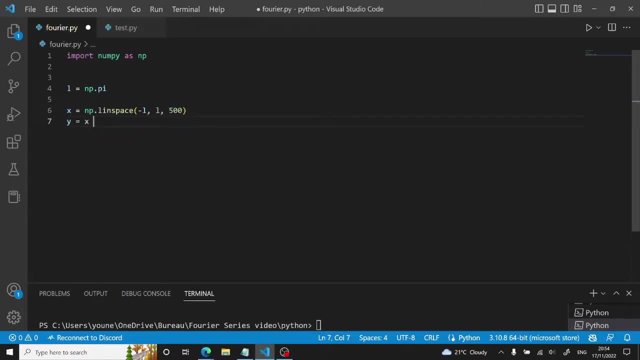 And then we define our y vector, which will be equal to x. let's say So: this stands for f of x. Okay, Now the first thing we can do is to compute our a0.. Okay, And we are going to go to our output. 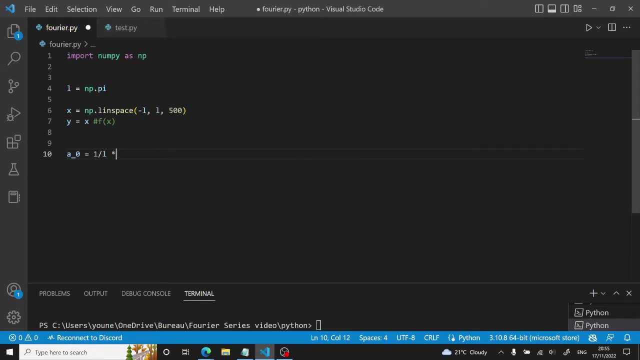 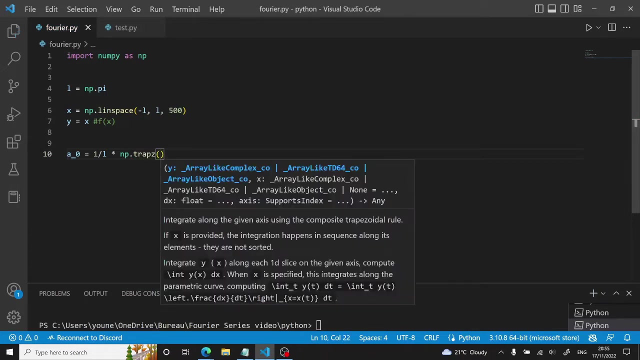 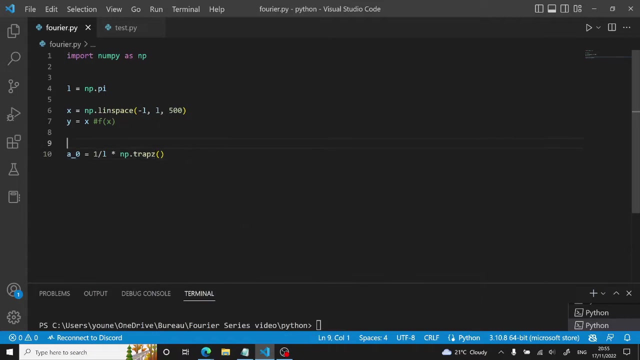 Okay, And then we will compute our l, which is equal to 1 over l, then times so with the integral. One way to compute an integral is with the numpytrapstraps method. Like so, So traps stands for trapezoidal, which is a numerical way to approximate an integral. 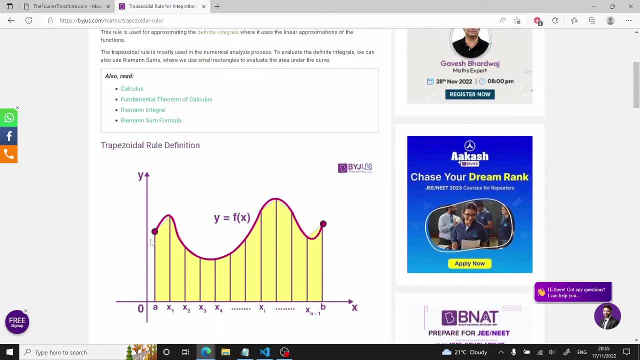 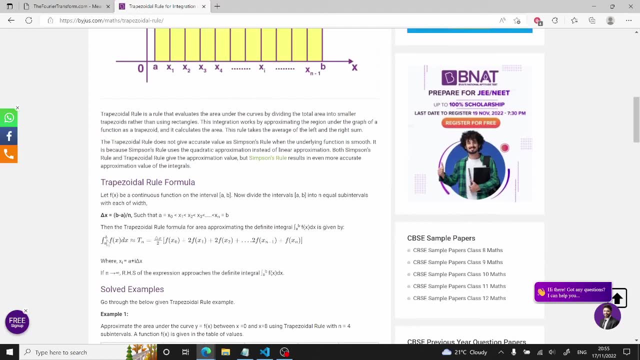 And I prepared here some estimates. Okay, So we are going to go to the trapezoidal Yes, a site where it can summarize what this method is about. like you can see here, you can approximate this integral by computing the value of the function at each point: x0, x1, x2 and so on. 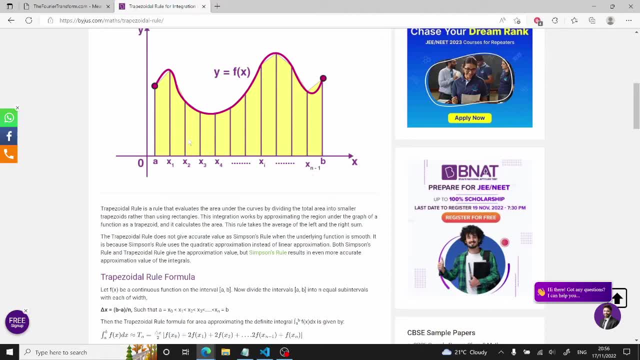 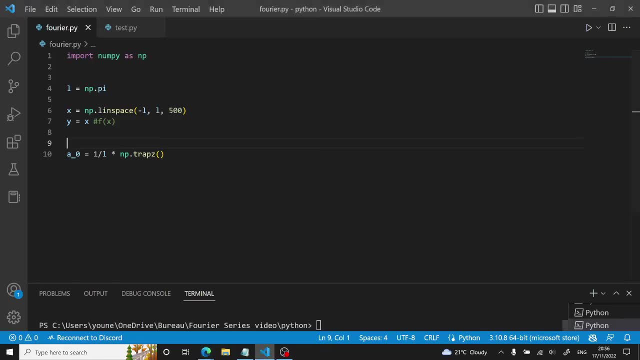 and then it is divided into n intervals, and the step of the intervals is denoted with dx. okay, so here it will be y. so this is the thing we want to integrate. and then it's x here, and then the number of intervals. we can set it to a hundred intervals. so this is the. 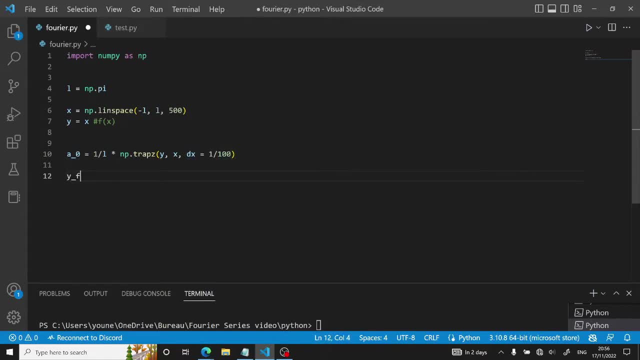 length of each interval. then we can initialize our self-generated Fourier series. okay, so this will be equal to numpy dot zeros having the length of x, and then we will add a zero over two, like so. so we have our first element of the series Fourier. now we need the other n elements. 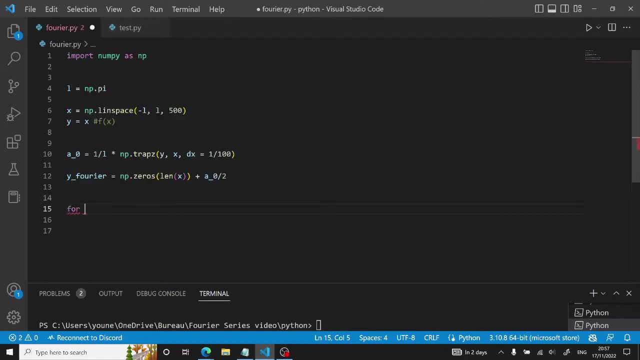 to do so, we will generate a for loop. so for n, in range of one until a hundred intervals. all right, so for now we will give it a whole sentence, but we have to start with x. that will laad Lars De ASMR to calculate the set x viele times per set. 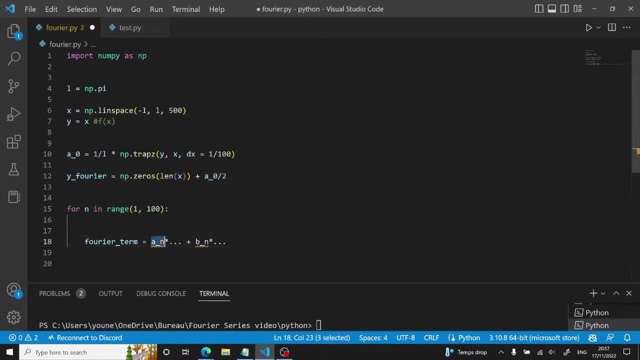 length. okay, so let's say i use less sum x200, so this will compute a hundred terms of the Fourier series. so the Fourier term will be equal to a n times something- oops, plus bn times something. so we have first to generate our a, n and bn. so we will do this right now. okay, this will be 100 MHz of information. Rozette will be 20.00 of遠обыling. this consists of two sets of terms. 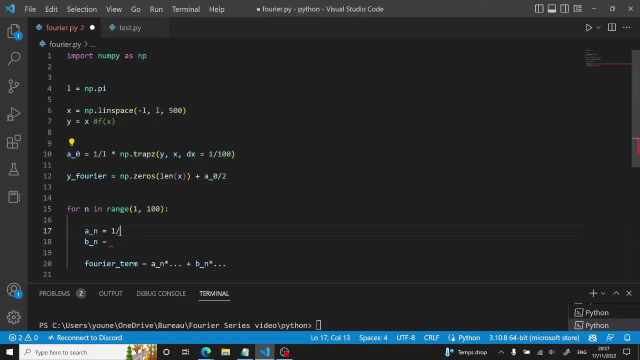 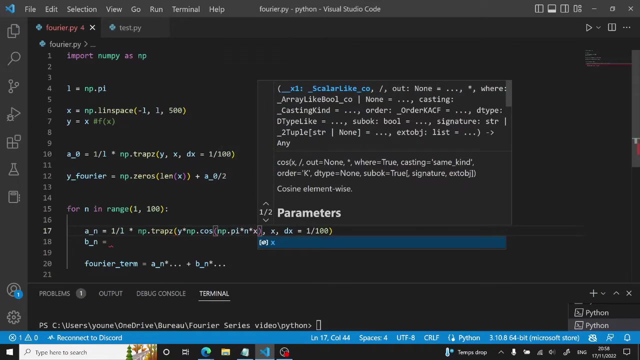 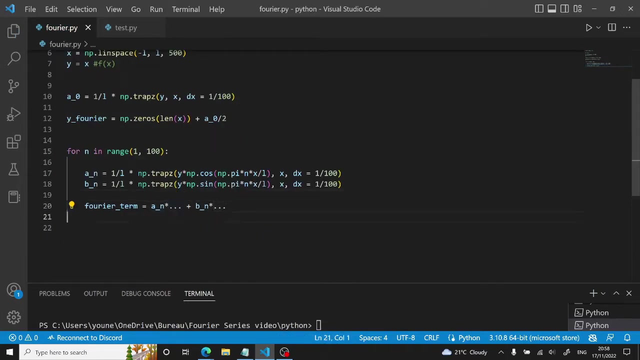 be equal, similarly to a0. uh, just copy this right here, and then here it's: y, then times np, dot, cos of np, dot, pi, times n, and then times x over l. all right, so this is the a? n, how we defined it, and then it's the same for bn, just modifying this with a sign. now the fourier term is a? n, and then 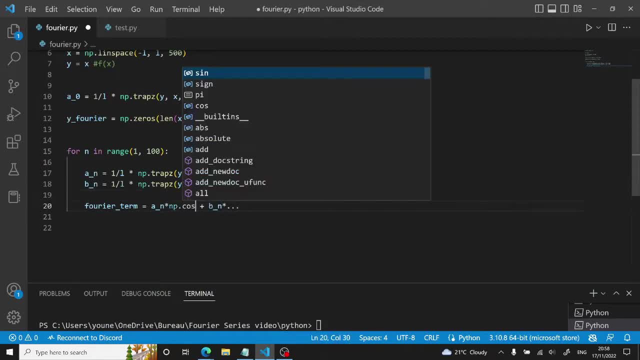 it's times np, dot, cos it's exactly the same expression right here, so we will copy this. and it's here npsign, and we will just copy it again. okay, so we have our fourier term. now we will add this vector right here. we can use the numpyadd method, so y fourier is equal to numpyadd. 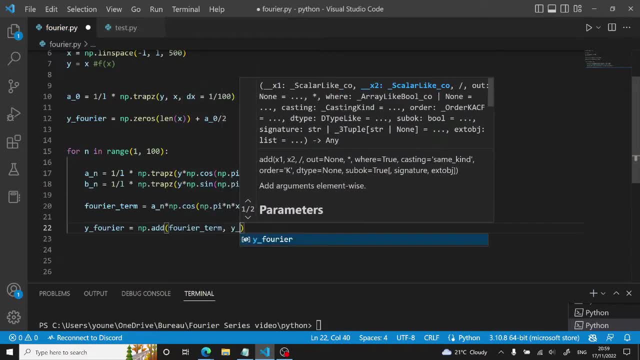 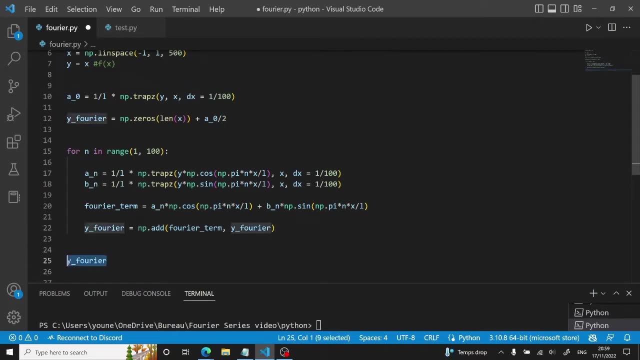 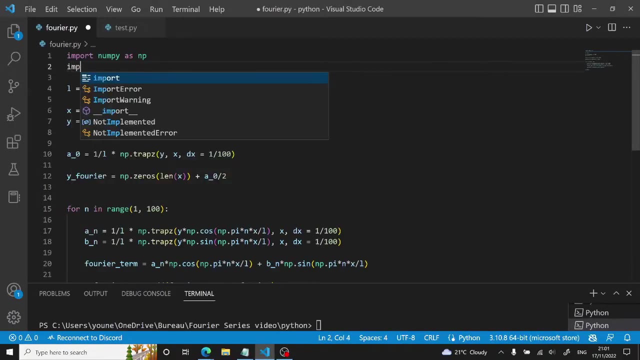 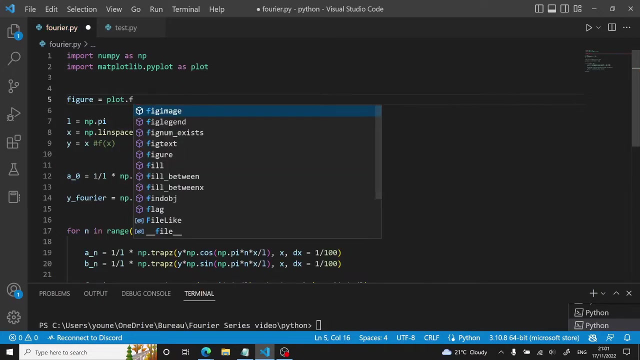 of fourier term: y dot fourier. okay, and then basically now we have our fourier series right here. okay, now we won't display our plots, so we will import matplotlibpiplot and then as plot we will create our figure. so figure is equal to plot dot figure. 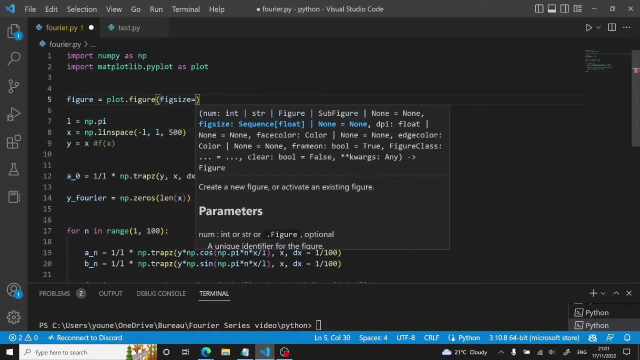 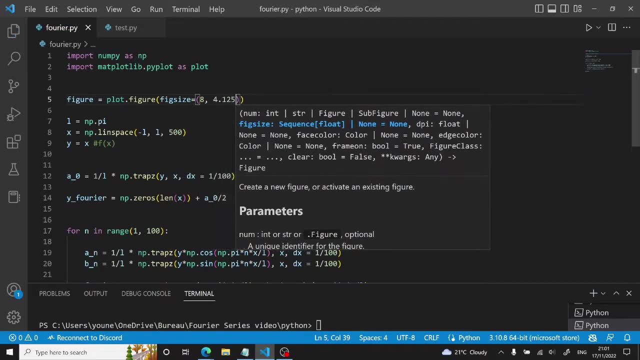 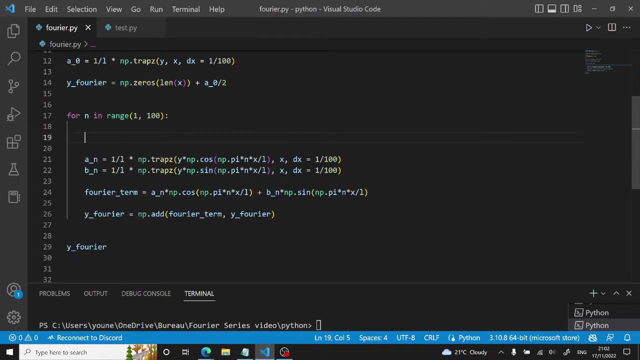 like so, and then you have inside, the fig size will be equal to eight, and then four dot one, two, five, okay, and then we will first display our y fourier and then compute it, because we already computed it here. so we will start by displaying and then, to do so, we are going to create axis, so axis. 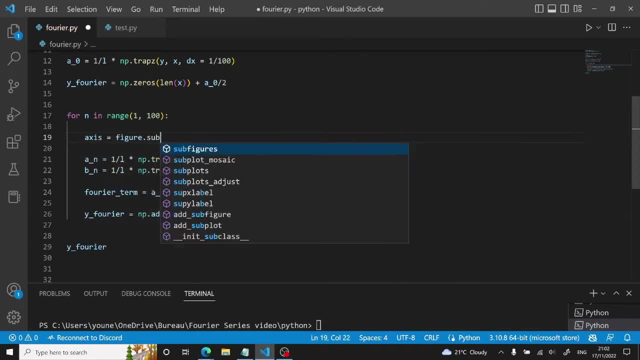 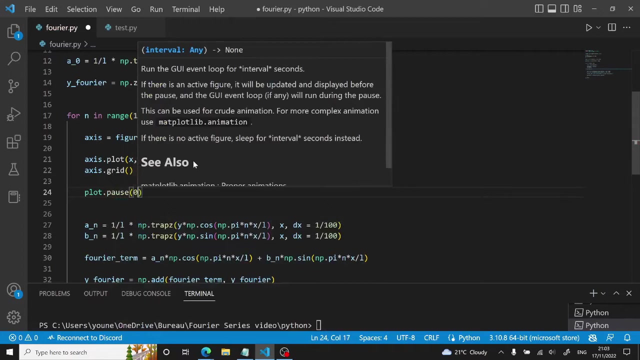 is equal. figure dot, subplots, okay, and then we will add a axis dot plot. we can just say x, then y of fourier. we can also add a grid, let's say so: axis dot grid, we have to pause it. plot dot pause, let's say of 0.05 seconds. we also have to draw it all right and then finally we'll. 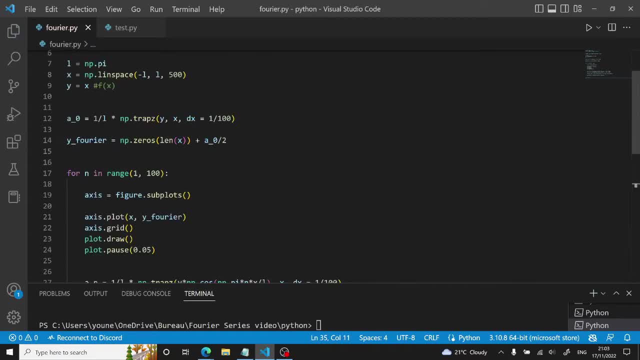 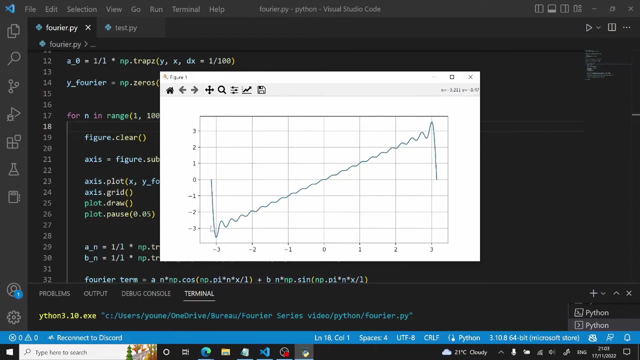 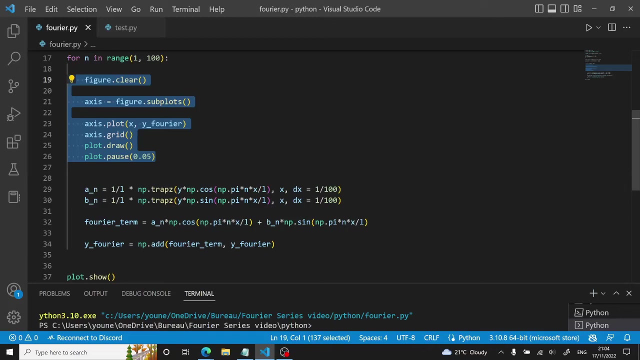 add a plot dot show. now we have to clear each time the figure or the axis. we will add a figure that clear. okay, then we run this. so you can see. this is our the evolution of the fourier series. now let me change this a little bit and make it a bit more clear and visually static. so i'll be right back. 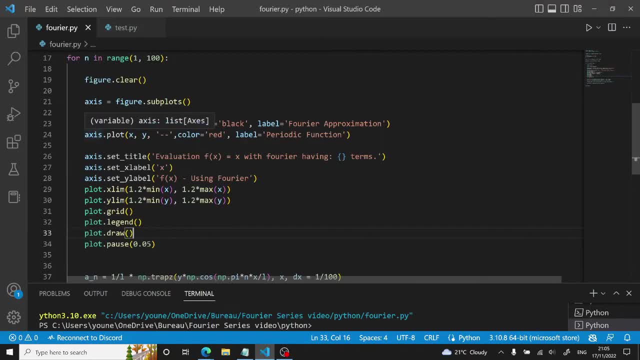 okay, so here i am back and the things i changed. so i add the color and then a label. here i also add another plot of the y so we can compare the actual function and the fourier generated series with a color of red and then a label of periodic function and some. 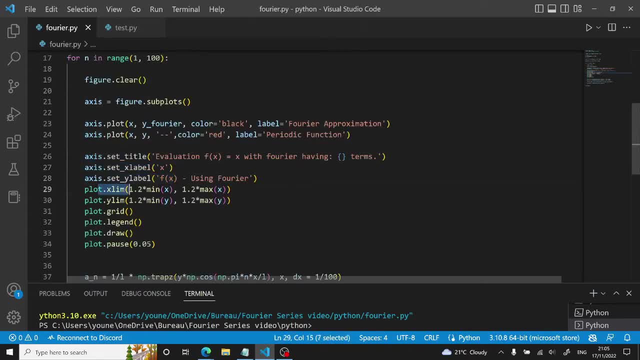 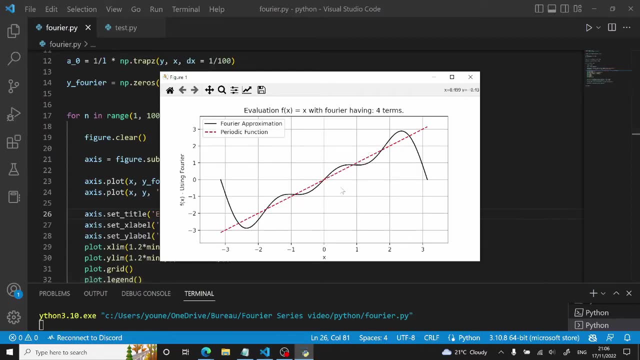 titles x, labels y and then the limits of the axis. all right, now you can see the numbers of terms increasing and then the more the number increases, the more we get closer to this function, this periodic function we generated. so now we want to know how actually close we are to this function. so to y equals x. 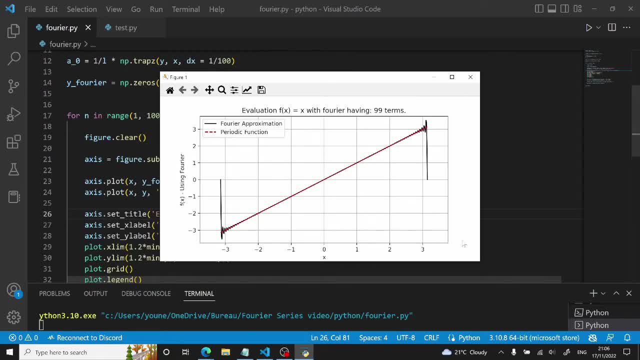 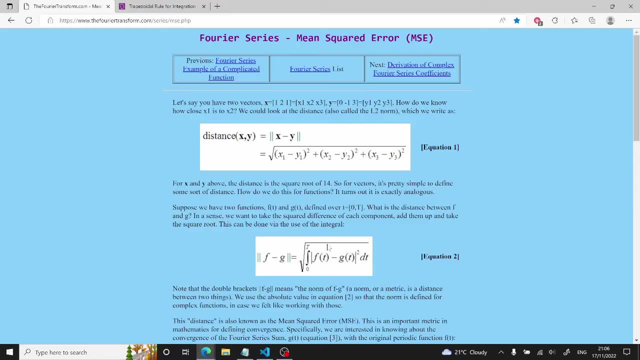 one way to do so is to compute the error of it. and to compute the error found that there is this notion right here, which is the mean squared error, where you can describe the similarity of f and g by computing this right here. so we will try and do this in visual studio code. 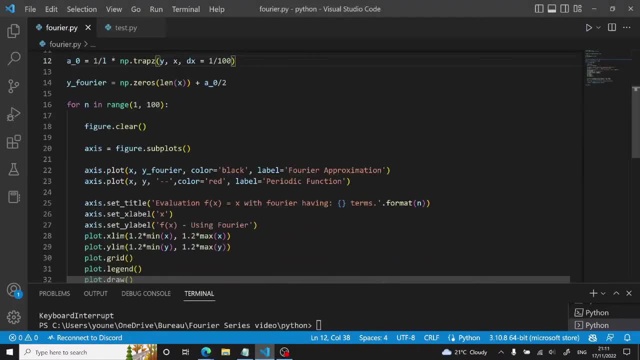 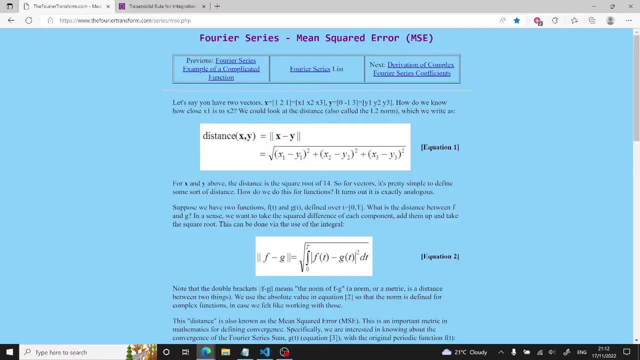 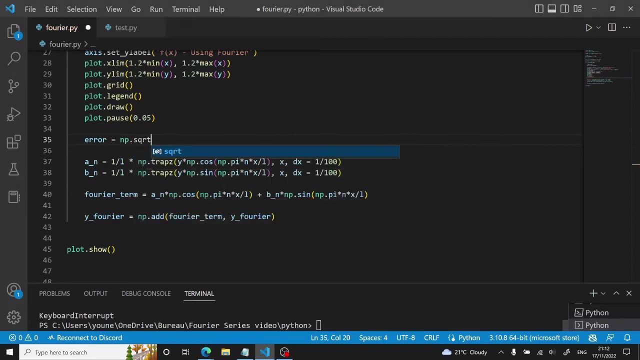 okay, so now we want to compute the error and we will create a new variable called error, and then, as you can see here, we have first to square root all of it, so it's going to be a numpy dot sqrt of something we need to square root: the integral. 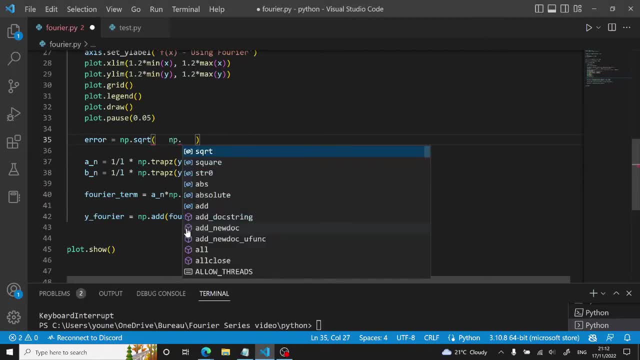 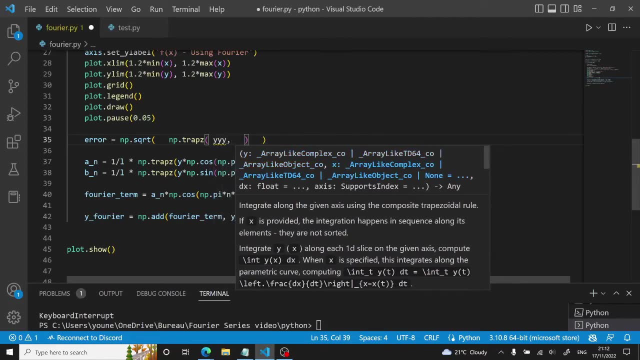 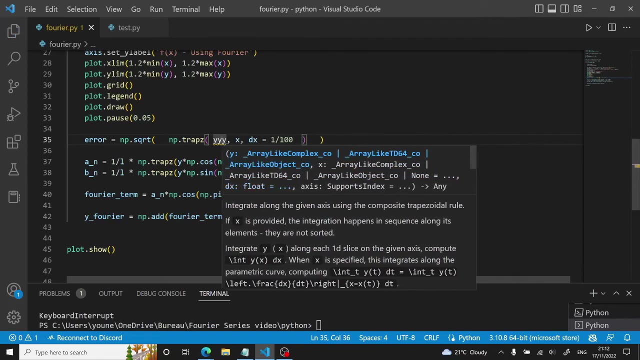 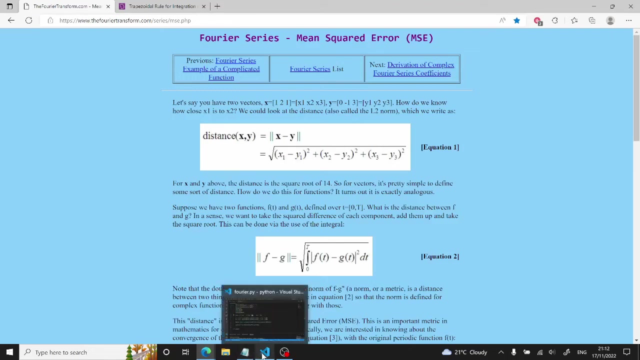 of this. so we are going to use the numpy dot traps again with it. then let's say: it's here, it will be y and then x. then dx is equal to 1 over 100. so now this y right here is in reality this expression right here. so it's the something. 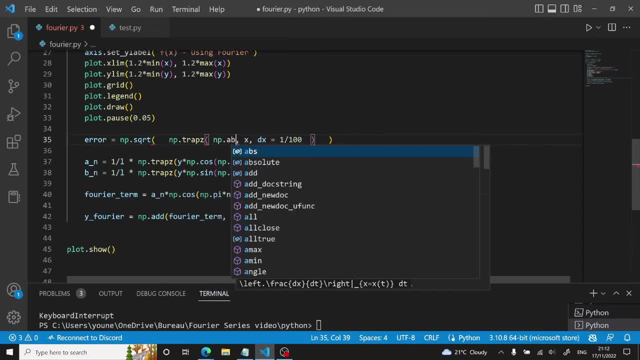 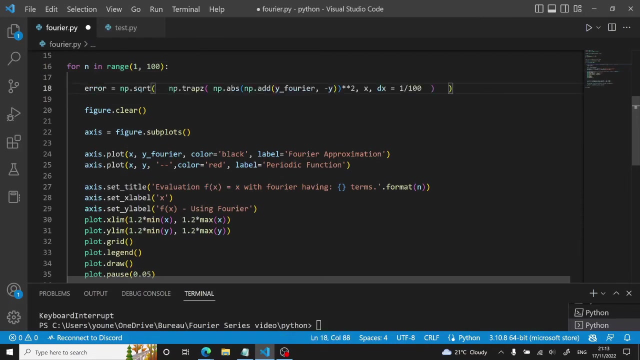 abs. so it's numpy dot abs of something squared. we are going to do numpy dot, add y, fourier, then minus y, like so make this one right here at the above, so we can also display it here in the title like so, and then we will do a, let's say error like so: okay, so we should. 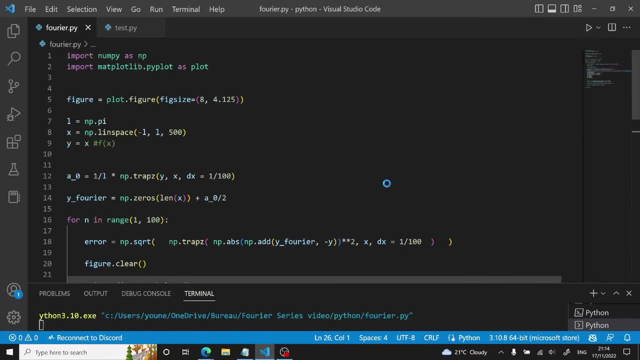 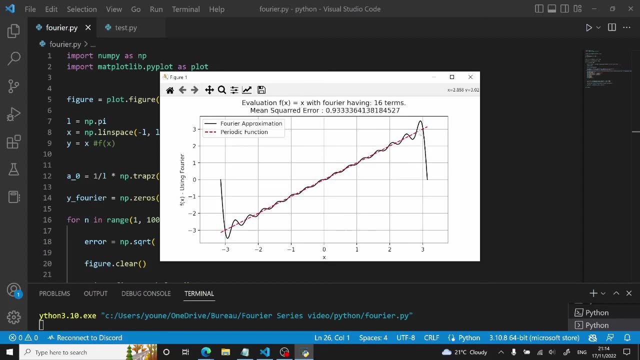 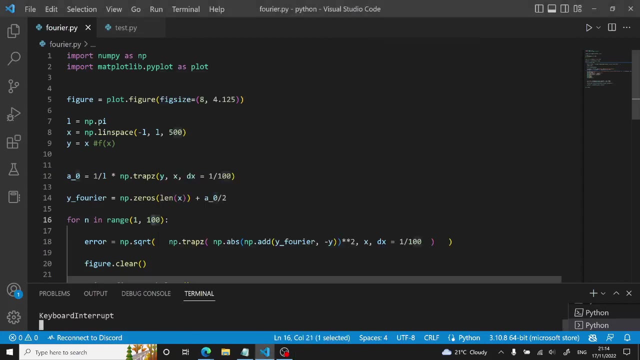 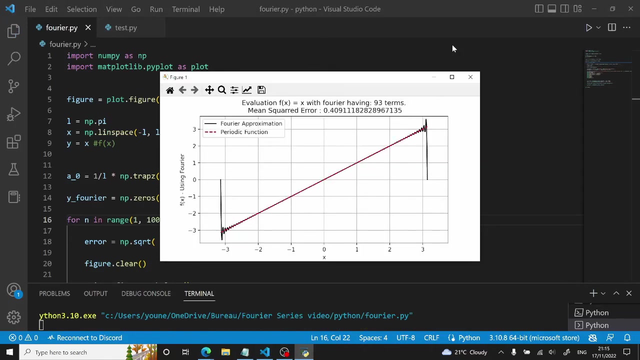 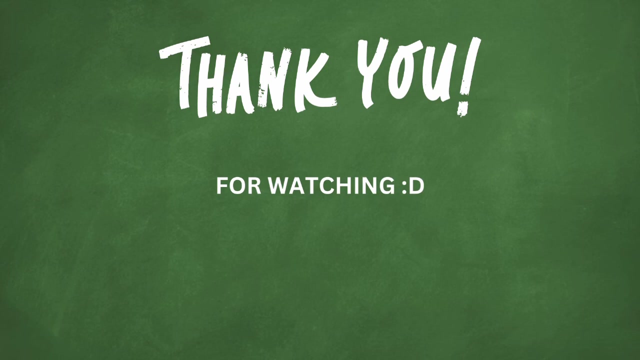 have everything. let's try run our code. so, yeah, you can see here the fourier series and it's evolving. then, each time it's evolving, you can see the error decreasing and then, well, we can take right here and then add thousand. so, yeah, thank you for watching this video. this has been my video of this. 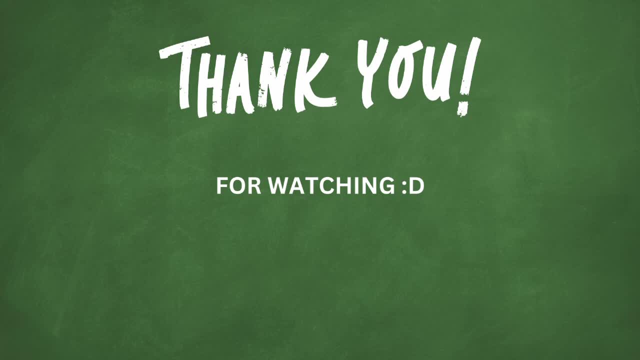 uh channel. i really enjoy making them, so uh consider subscribing if you want to see more and see ya.